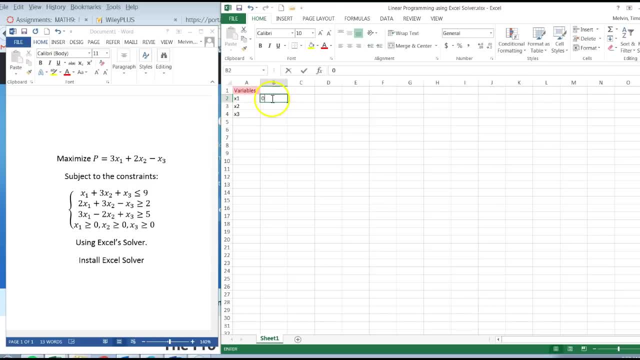 and x1,, x2,, x3, and, just to start this off, I'm going to make them all zero. Make them whatever you want, but I'll make them zero. all right here. The next thing I'm going to type in is the objective. So the objective in this. 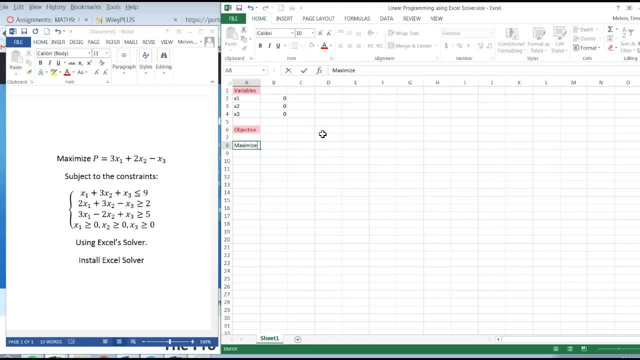 example, you want two maximums and now I'm going to enter in this function P. So I'm to start with an equals 3 times x1. I'm going to click on the cell b2 up here, plus 2 times x2, and the values can go in b3 finally minus x3, which is b4 in my 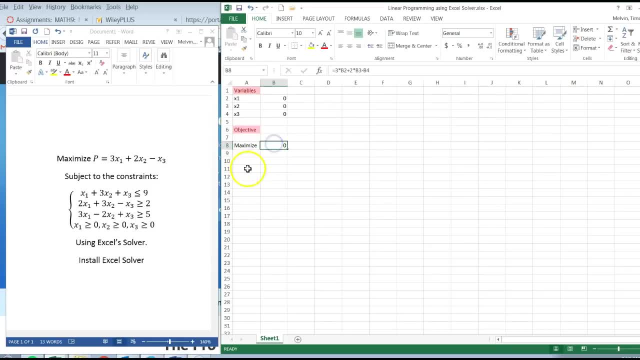 spreadsheet. I'm going to click on enter and that's going to be 0, and then I want to add in the constraints. all right, so the constraints, I'm going to go right over here, all right. the number of constraints: two, three, four, five, six. there are six constraints total and I'm going to do quality just to set up the. 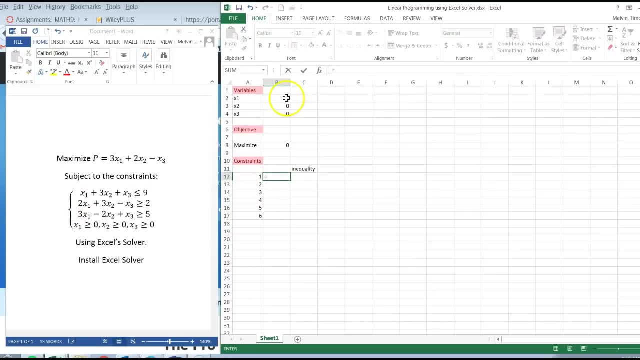 first constraint and then I'm going to add in the constraints and then I'm going to add in the constraints. all right, so the first constraint: start with equal sign. first constraint: start with equal sign. first constraint: start with equal sign. it's going to be x1 plus 3 times x2 plus. 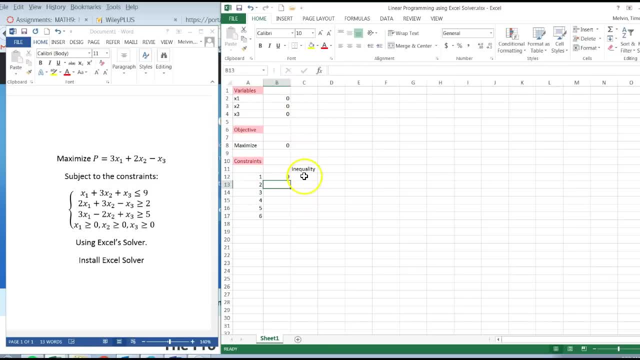 it's going to be x1 plus 3 times x2 plus. it's going to be x1 plus 3 times x2 plus x3. click on enter. and inequality: that is x3. click on enter. and inequality: that is x3. click on enter. and inequality, that is a less than or equal to, and then I'm. 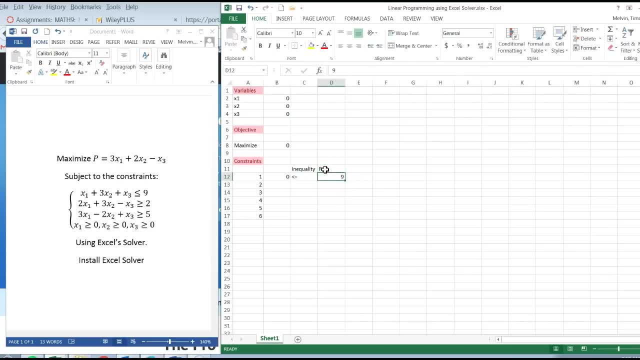 a less than or equal to, and then I'm a less than or equal to, and then I'm gonna click on a 9 right here. I'll type gonna click on a 9 right here. I'll type gonna click on a 9. right here, I'll type in our H? s or right hand side, or the: 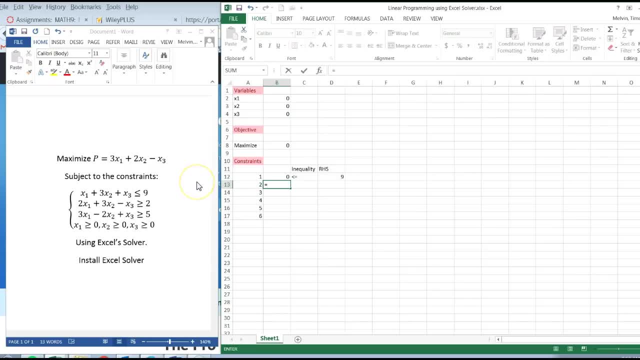 in our H? s or right hand side, or the in our H? s or right hand side, or the second constraint. I want to type it in second constraint. I want to type it in second constraint. I want to type it in. I'm going to do equals 2 times x1 plus. 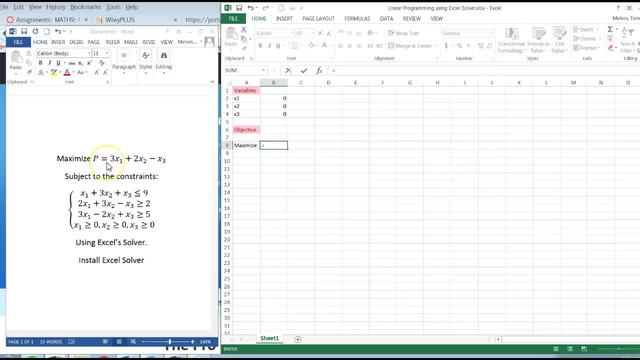 function P. so I'm gonna start with an equals 3 times x1. I'm gonna click on the cell b2 up here plus 2 times x2, and the values can go in b3 finally, minus x3, which is b4 in my spreadsheet, I'm gonna click on enter and that's going to be. 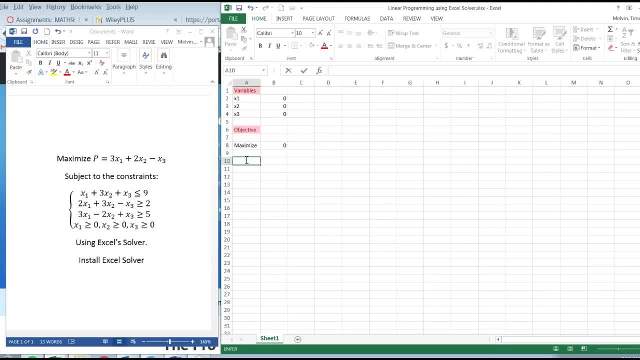 0. and then I want to add in the constraints. all right, so the constraints I'm going to go out over here, all right. the number of constraints: two, three, four, five, six. there are six constraints total and I'm gonna do equality. just to set up the first constraint, start with equal sign. it's. 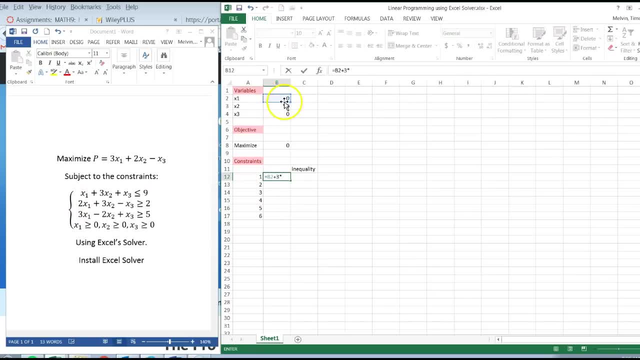 going to be x1 plus 3 times x2 plus x3. click on enter and inequality, that is, a less than or equal to, and then I'm going to click on a 9 right here I'll type in our HS for a right-hand side, for the second constraint, I want to type it in: 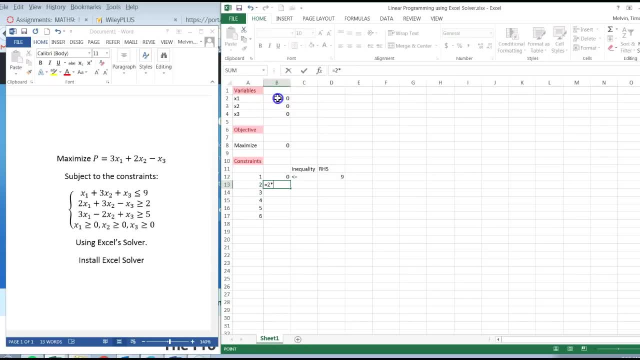 I'm going to do it. equals 2 times x 1, plus 3 times x 2 and then minus x 3 enter and that's going to be a greater than or equal to right-hand side would be 2. third constraints right here. equals 3 times x 1. 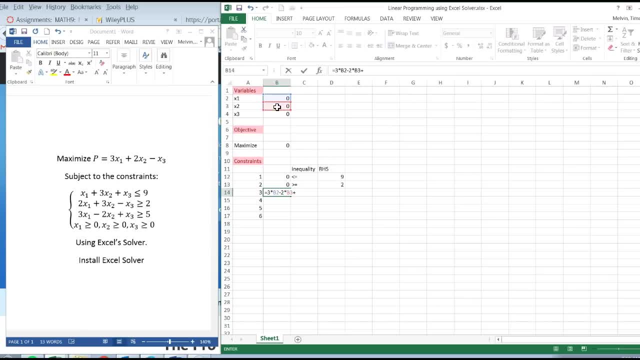 minus 2 times X 2 plus X 3. click on enter and that's going to be greater than equal to 5. all right, so there are. there's a shortcut on these last constraints. I'll show you in a second, but just in case they're not all greater. 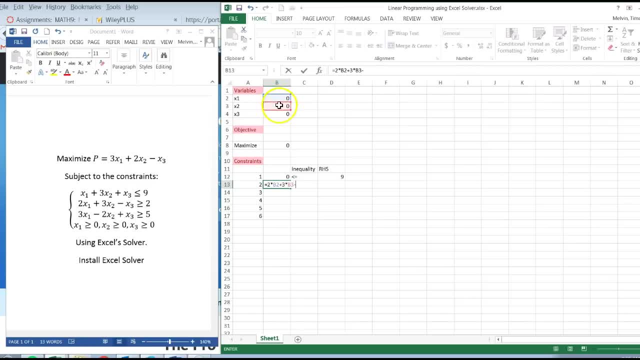 I'm going to do equals 2 times x1 plus. I'm going to do equals 2 times x1 plus 3 times x2 and then minus x3, click on 3 times x2 and then minus x3, click on 3 times x2 and then minus x3, click on enter, and that's going to be a greater. 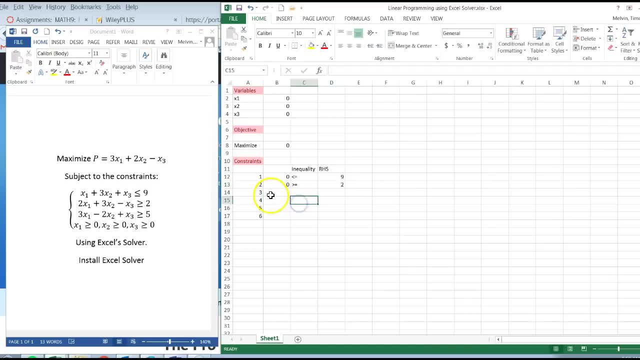 enter and that's going to be a greater enter and that's going to be a greater than, or equal to right-hand side will be than, or equal to right-hand side will be than or equal to right-hand side will be: 2 third constraints. right here equals. 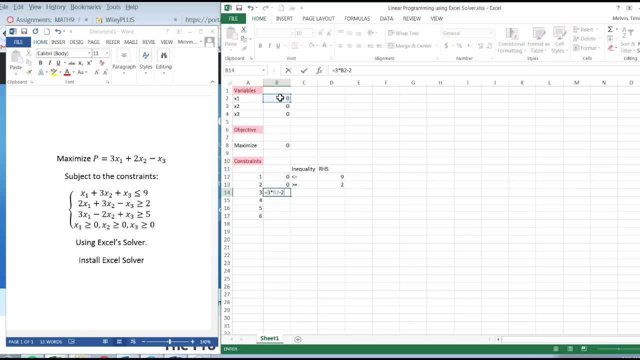 2 third constraints right here equals 2 third constraints right here equals 3 times x1 minus 2 times x2 plus x3. 3 times x1 minus 2 times x2 plus x3. 3 times x1 minus 2 times x3. click on enter and that's going to be. 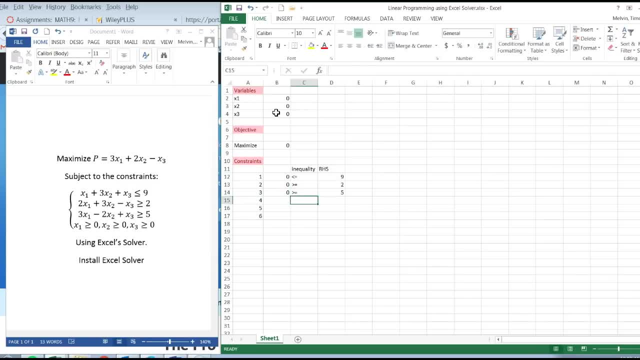 click on enter and that's going to be click on enter and that's going to be greater than equal to 5- all right. so greater than equal to 5, all right. so greater than equal to 5, all right. so there are. there's a shortcut on these. there are. there's a shortcut on these. there are. there's a shortcut on these last constraints. I'll show you in a last constraints. I'll show you in a last constraints. I'll show you in a second, but just in case they're not all. second, but just in case they're not all. 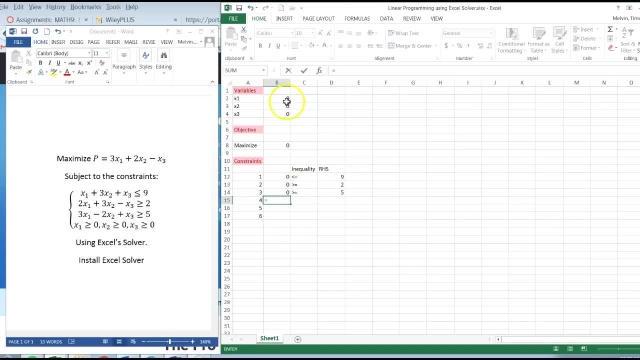 second, but just in case they're not all: greater than you can always add these. greater than you can always add these. greater than you can always add these here. this is just that. x1 it's greater here. this is just that x1 it's greater here. this is just that x1 it's greater than or equal to 0. it's gonna be equal. 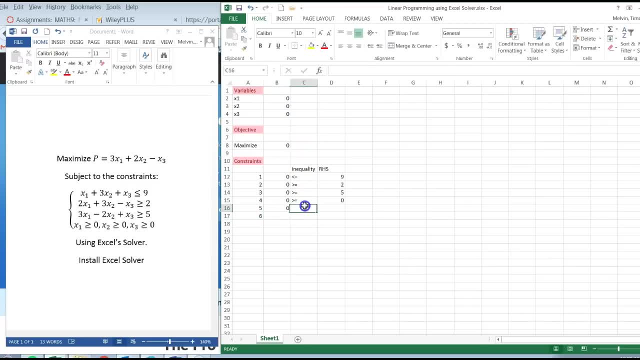 than or equal to 0. it's gonna be equal than or equal to 0. it's gonna be equal to x2. it's greater than or equal to 0 to x2. it's greater than or equal to 0 to x2. it's greater than or equal to 0. and lastly, I've got x3. excuse me, equals. 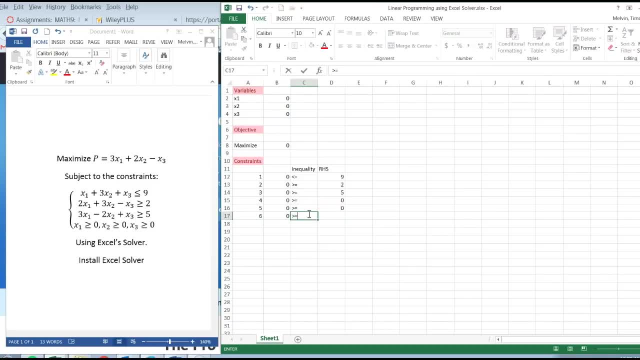 and lastly, I've got x3- excuse me, equals. and lastly, I've got x3- excuse me, equals. x3- enter greater than or equal to 0- okay. x3- enter greater than or equal to 0- okay. x3- enter greater than or equal to 0- okay. so now I have this set up, I don't. 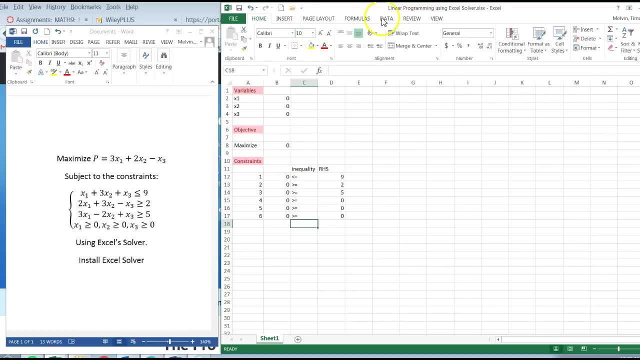 so now I have this set up, I don't. so now I have this set up, I don't really need this file anymore. but I'm really need this file anymore. but I'm really need this file anymore. but I'm gonna go over to a solver. so the top for. 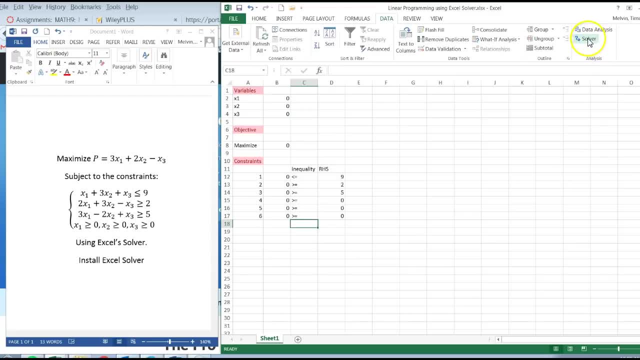 gonna go over to a solver, so the top for gonna go over to a solver. so the top for Excel: click on the data tab and then Excel click on the data tab and then Excel click on the data tab and then towards the right. this should have been. 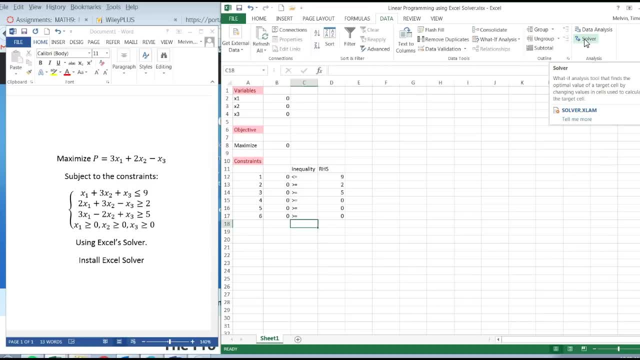 towards the right. this should have been towards the right. this should have been added already. if not, make sure to go to added already. if not, make sure to go to added already. if not, make sure to go to file add-ins. all right, and I'm gonna file add-ins. all right, and I'm gonna. 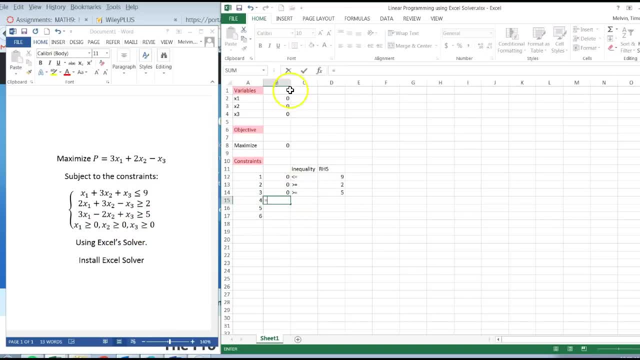 than you can always add these here. this is just that X 1, it's greater than or equal to 0, it's going to be equal to X 2: it's greater than or equal to 0. and lastly, I've got X 3, excuse me, equals X 3. enter greater than or equal to 0. 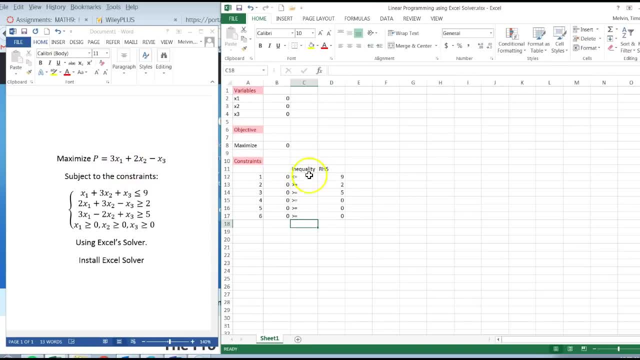 okay, okay, okay, okay. so now I have this set up. you don't really need this file anymore. but I'm gonna go over to a solver. so the top for Excel, click on the data tab and then towards the right. this should have been added already. if not, make sure to go to. 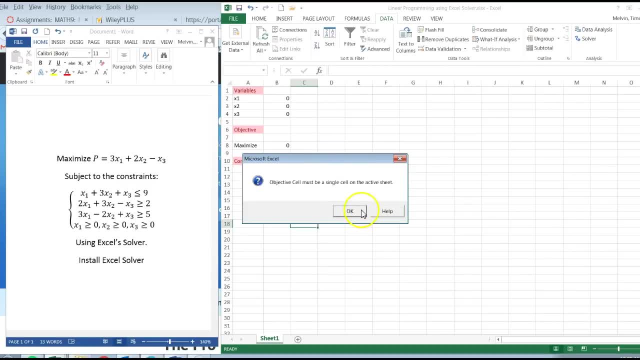 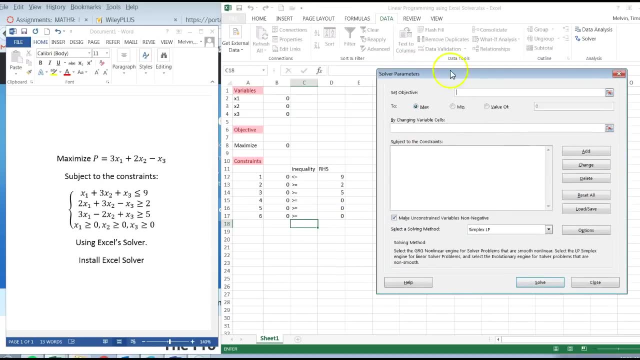 file add-ins. all right, and I'm gonna restore all. that's first time using solver. this is what you should see right here: set objective. I'm gonna click on the objective right there. it's just a zero. key is a dollar B, dollar 8, and we want to maximize this and by changing cells are going to be three. 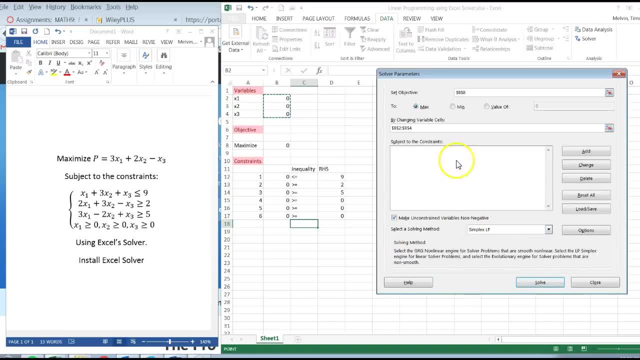 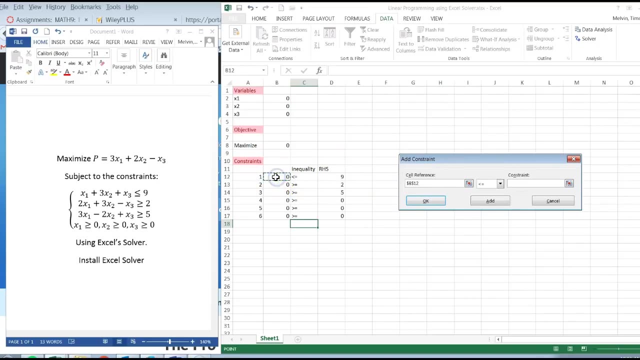 verbs. so I've got set objective to max in this example by changing cells, my variables, and now we need to go down here and add my constraints. so I click on the Add button, add the constraints. the first constraints right here- and this is a less than or equal to, the right-hand side, is a 9. I'm going to 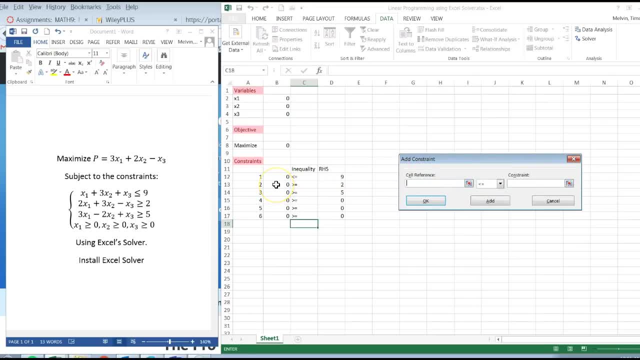 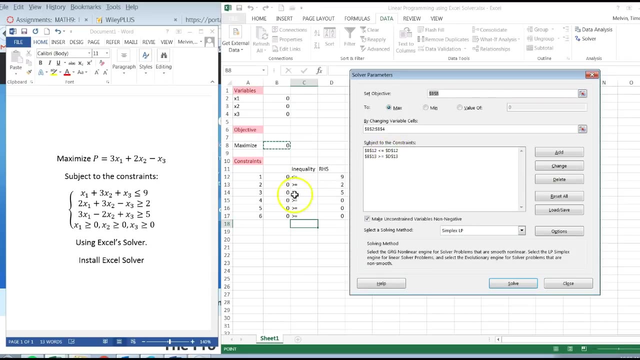 click on add the second constraint. click on here now this is a greater than or equal to, and click on the to make sure you keep track of each constraint as you go. I click OK, I've added two of them. I got to add the other four, so I adds. 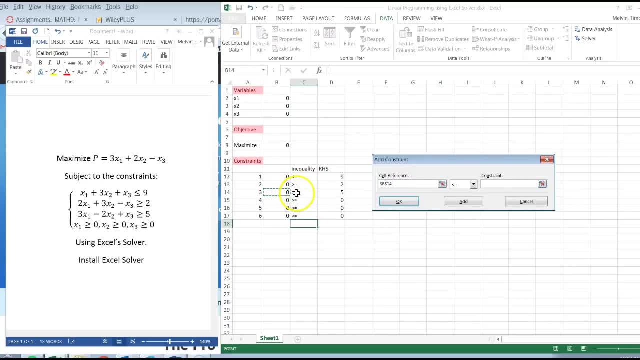 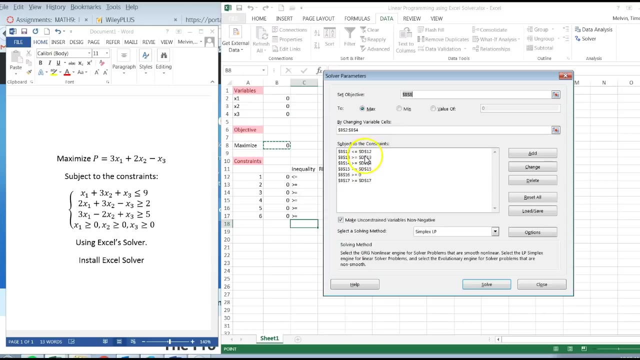 third constraint: click on the constraint greater than or equal to, and the constraint would be five: add. fourth constraint: greater than equal to zero: add. fifth constraint: greater than equal to zero: add. and the last constraint is the third variable: x3 is going to be greater than equal to zero. click OK, notice. right here I have all my 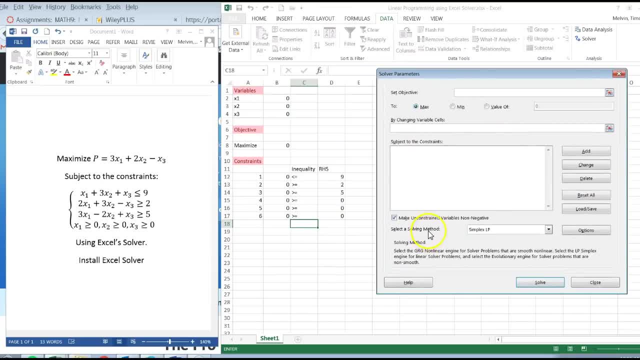 file add-ins. all right, and I'm gonna restore all that's first time using. restore- all that's first time using. restore all that's first time using solver. this is what you should see, right solver. this is what you should see, right solver. this is what you should see right here: set objective. I'm gonna click on. 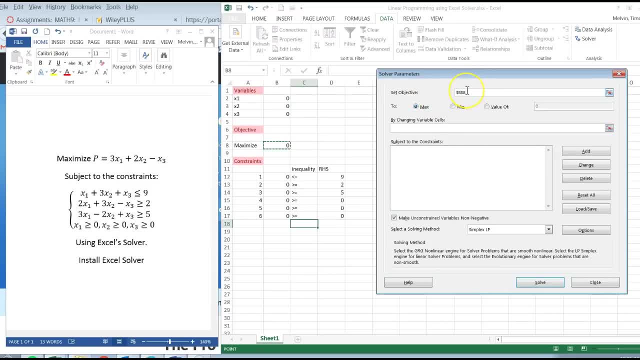 here set objective. I'm gonna click on here set objective. I'm gonna click on the objective: right there, it's just a. the objective right there, it's just a. the objective right there, it's just a zero. he is a dollar, be dollar eight and zero. he is a dollar, be dollar eight and. 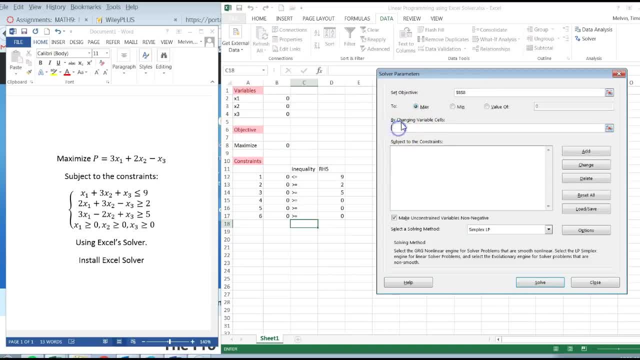 zero, he is a dollar, be dollar eight. and we want to maximize this. and by changing, we want to maximize this. and by changing, we want to maximize this. and by changing. cells are gonna be three verbs, so I've. cells are gonna be three verbs, so I've. 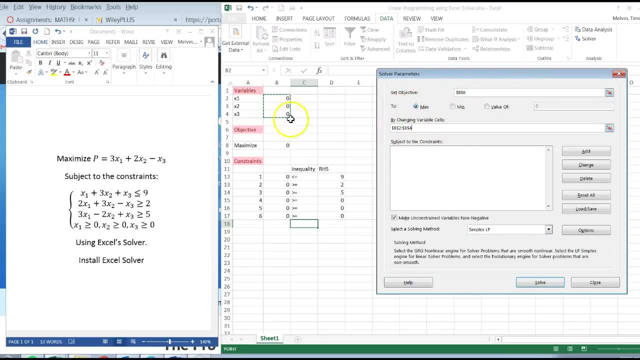 cells are gonna be three verbs. so I've got set objective to max in this example, got set objective to max in this example, got set objective to max in this example by changing cells- my variables, and now by changing cells, my variables, and now by changing cells, my variables. and now we need to go down here and add my. 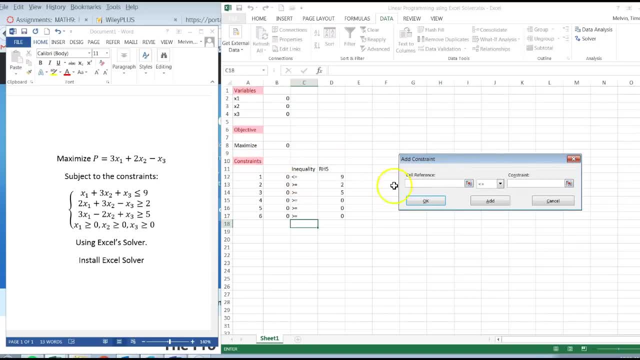 we need to go down here and add my. we need to go down here and add my constraints. click on add button. add the constraints. click on add button. add the constraints. click on add button. add the constraints: the first constraints, right constraints, the first constraints, right constraints, the first constraints right here. and this is a less than or equal to: 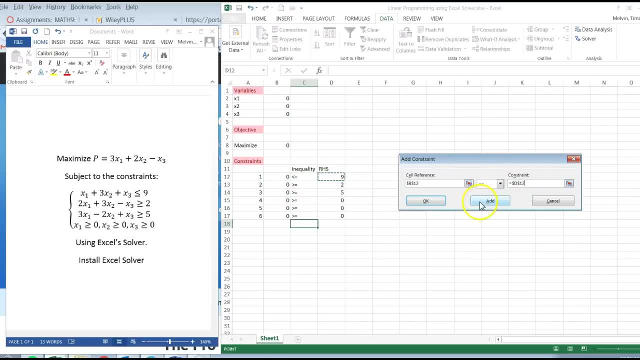 here and this is a less than or equal to here, and this is a less than or equal to. the right-hand side is a 9. I'm gonna. the right-hand side is a 9. I'm gonna the right-hand side is a 9. I'm gonna click on add the second constraint. 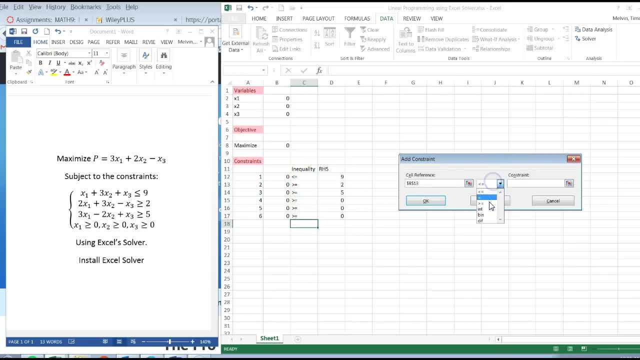 click on add the second constraint. click on add the second constraint. click on here now. this is a greater than. click on here now. this is a greater than: click on here now. this is a greater than, or equal to, and click on the to make. or equal to and click on the to make. 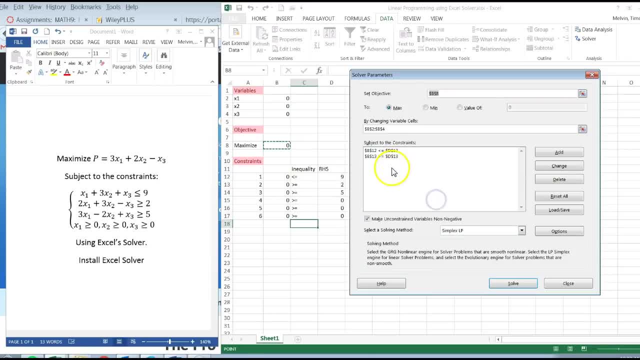 or equal to, and click on the to make sure you keep track of each constraint. sure you keep track of each constraint. sure you keep track of each constraint as you go, I click OK. I've added two of. as you go, I click OK, I've added two of. 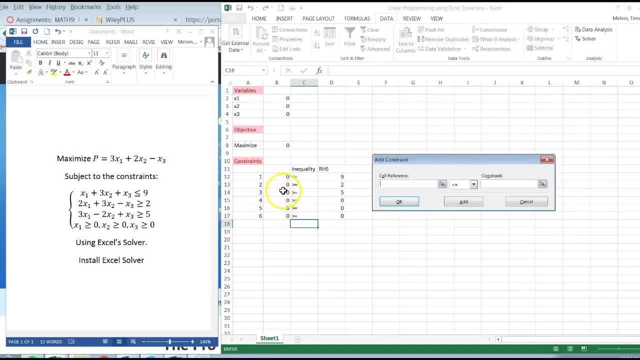 as you go, I click OK, I've added two of them. I got to add the other four, so adds them. I got to add the other four, so adds them. I got to add the other four, so adds third constraint. look on the third constraint. look on the. 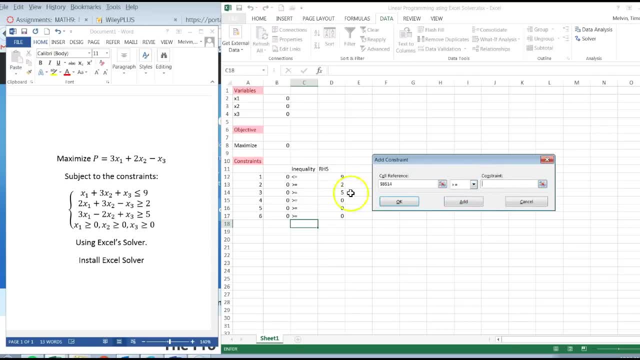 third constraint: look on the constraint greater than or equal to, and the constraint greater than or equal to, and the constraint greater than or equal to, and the constraint would be five. add fourth constraint would be five. add fourth constraint would be five. add fourth constraint greater than equal to zero. 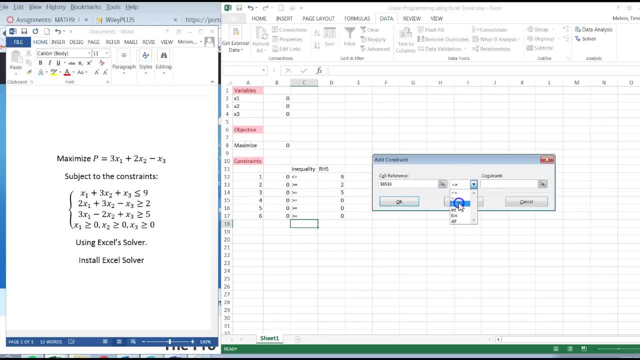 constraint greater than equal to zero constraint greater than equal to zero: add. fifth constraint greater than equal to add. fifth constraint greater than equal to add. fifth constraint greater than equal to zero add and the last constraint is zero add. and the last constraint is zero add. and the last constraint is the third variable. x3 is going to be. 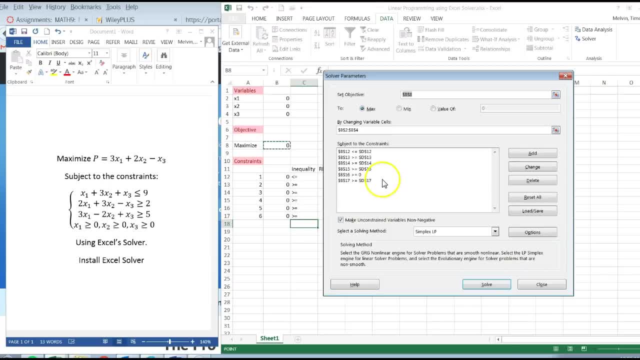 the third variable. x3 is going to be the third variable. x3 is going to be greater than equal to zero- click OK. greater than equal to zero: click OK. greater than equal to zero: click OK. notice right here. I have all my notice. right here, I have all my. 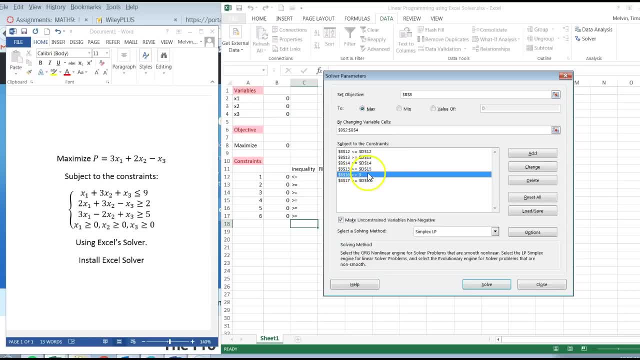 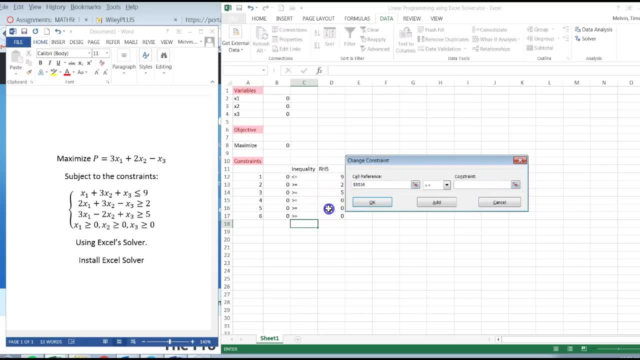 notice, right here I have all my constraints. let's see I should be okay. constraints. let's see I should be okay. constraints. let's see I should be okay with this zero. but I could click on the with this zero. but I could click on the with this zero. but I could click on the change right here and make this. so I got. 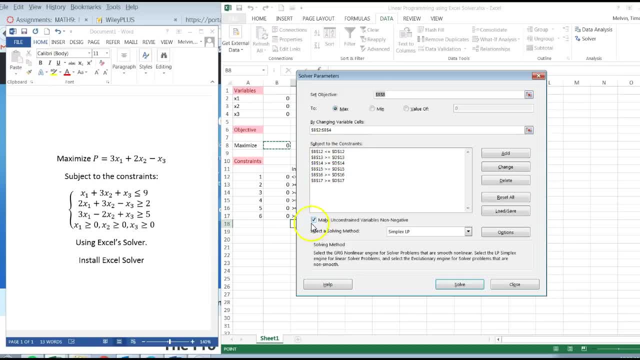 change right here and make this. so I got change right here and make this. so I got it all set up. now all my constraints, it all set up. now all my constraints are set up and, as I mentioned earlier, are set up. and, as I mentioned earlier, are set up and, as I mentioned earlier, there's a shortcut. you didn't have to do. 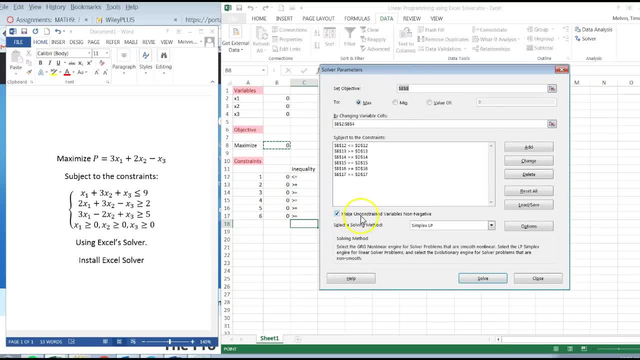 there's a shortcut you didn't have to do. there's a shortcut. you didn't have to do this bottom three constraints. because this bottom three constraints, because this bottom three constraints? because there is an option to make make. there is an option to make make. there is an option to make make unconstrained variables non-negative. but 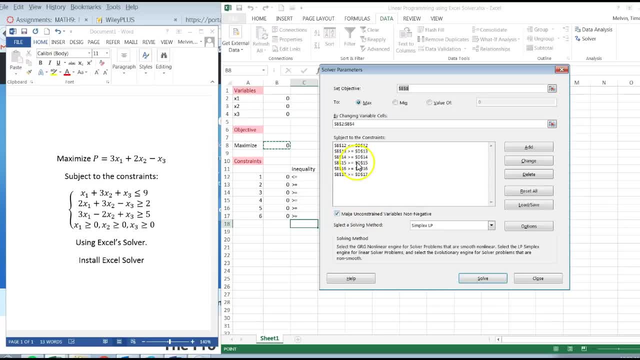 unconstrained variables: non-negative. but unconstrained variables: non-negative. but there could be some examples where the there could be some examples where the there could be some examples where the variables can be negative. so I like variables can be negative. so I like variables can be negative. so I like entering them in manually for selecting. 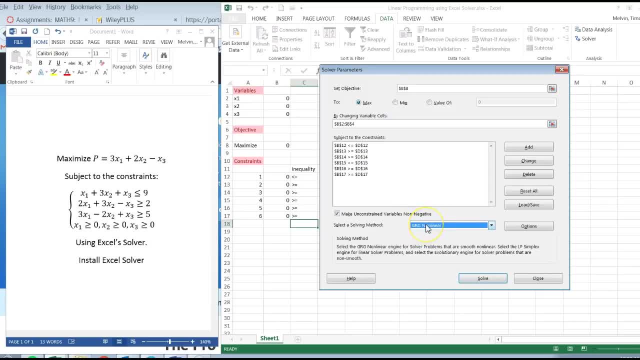 entering them in manually for selecting. entering them in manually for selecting an option at the bottom. you might you an option at the bottom, you might you an option at the bottom, you might you might set up to be nonlinear, you want to might set up to be nonlinear, you want to. 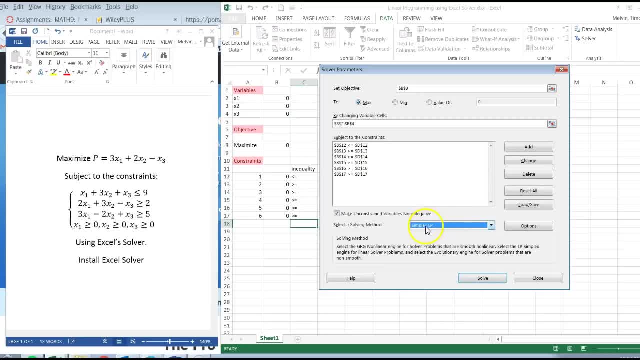 might set up to be nonlinear. you want to make sure this says simplex LP. use the. make sure this says simplex LP. use the. make sure this says simplex LP. use the simplex algorithm and then click on the simplex algorithm and then click on the simplex algorithm and then click on the solve button. and if you notice over here, 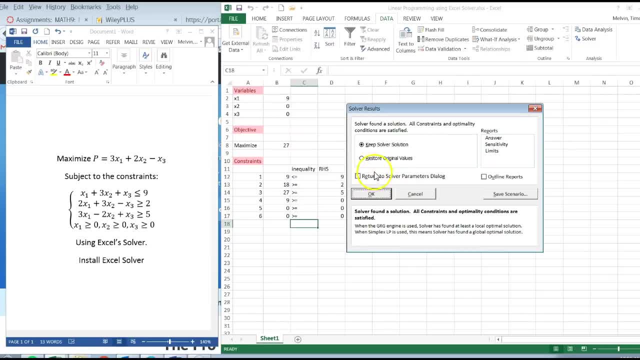 solve button. and if you notice over here, solve button. and if you notice over here, these values change: X 1 is 9 0 0. we these values change: X 1 is 9 0 0. we these values change: X 1 is 9 0 0. we can restore original values. I'll click on. 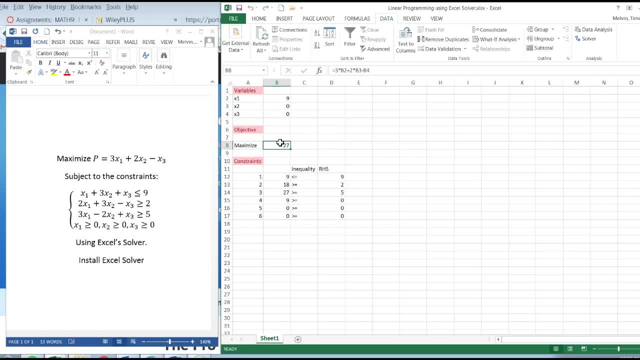 can restore original values? I'll click on. can restore original values? I'll click on OK, and here we have our solution. so OK, and here we have our solution. so OK, and here we have our solution. so the maximum value for this P is 27 max. the maximum value for this P is 27 max. 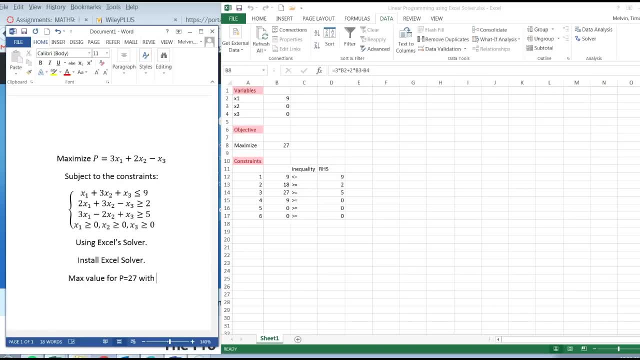 the maximum value for this P is 27. max value for P equals 27. with X 1 equals 9. value for P equals 27. with X 1 equals 9. value for P equals 27. with X 1 equals 9, X 2 equals 0, X 3 equals 0. so we have our. X 2 equals 0, X 3 equals 0, so we have our X 2 equals 0, X 3 equals 0, so we have our solution right here. solution right here.